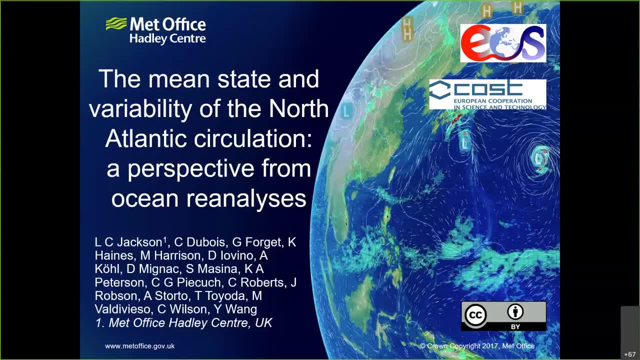 including research on variability, projections, influence of resolution and understanding stability and risks of a collapse. She has collaborated with various UK rapid projects and has been and has recent collaborations with the OSNAP community. She has also recently been working with the ocean reanalysis community and understanding how ocean reanalysis represent 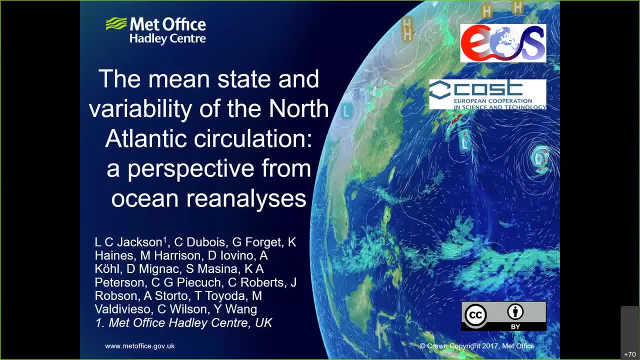 dynamics, which has led to her leading best paper presented today. So with that, go ahead, Laura. Okay, thank you, Jenny. The title of this talk is Mean State and Variability of the North Atlantic Circulation with Respect to Promotional Analysis, and this is based on a paper that's 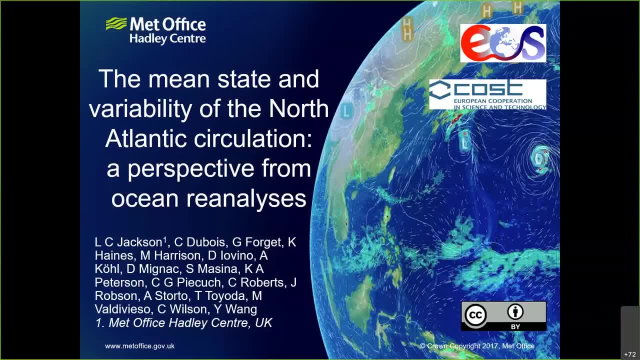 published end of last year as part of the USA AMOC virtual edition. I should say this paper originated actually from the reanalysis community rather than the AMOC community. So I previously published a paper which looked at the AMOC and our Met Office ocean reanalysis and ended up volunteering to organize this paper, which 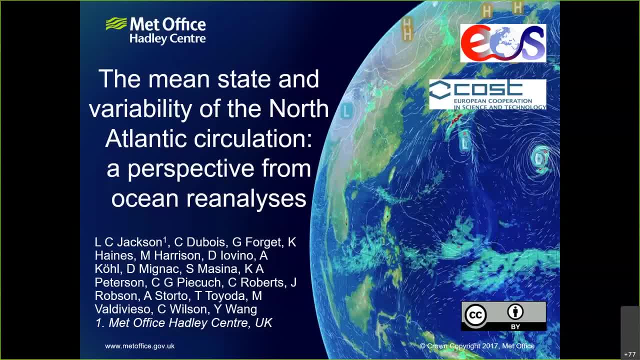 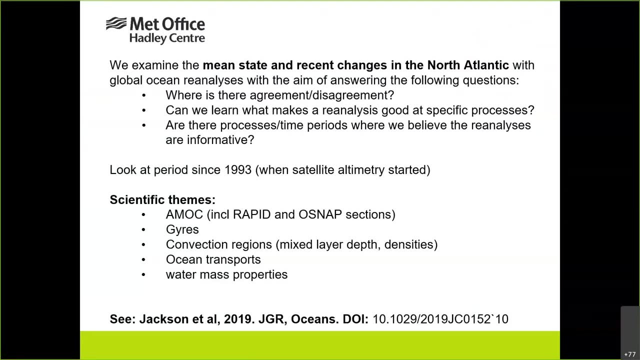 compares a number of different analyses. So this talk does differ from other talks in this series and that is it's a comparison paper rather than a review and it doesn't primarily focus on the AMOC. So the scope of this study: we examined the mean state and recent changes in the North 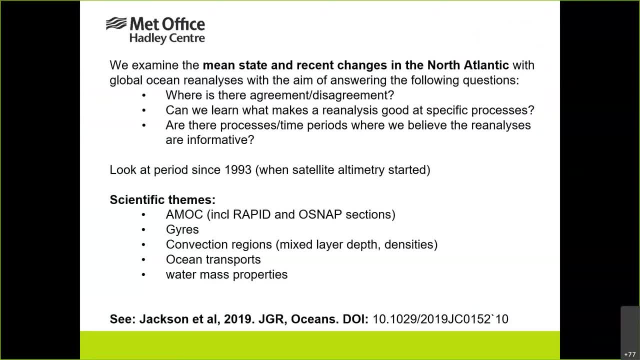 Atlantic, with global ocean reanalyses, with the aim of answering some questions. So where is there agreement and disagreement? Can we learn what makes a reanalysis good at specific processes? Are there periods where we believe the reanalysis are informative? In particular, we've looked at the period since: 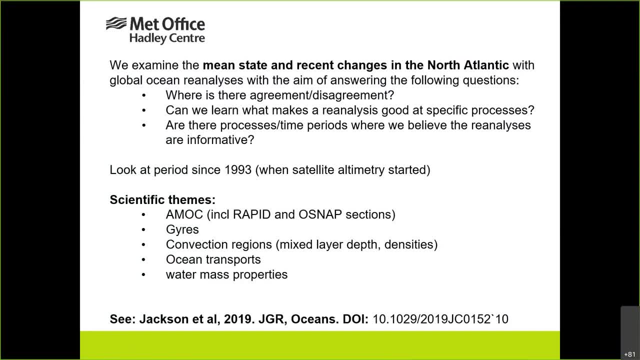 1993, which is probably the most recent period, Okay, Which is when our satellite has literally started since. that's when these reanalyses have been best constrained. So scientific themes. so you looked at the AMOC, That's the rapid and OSNAP. 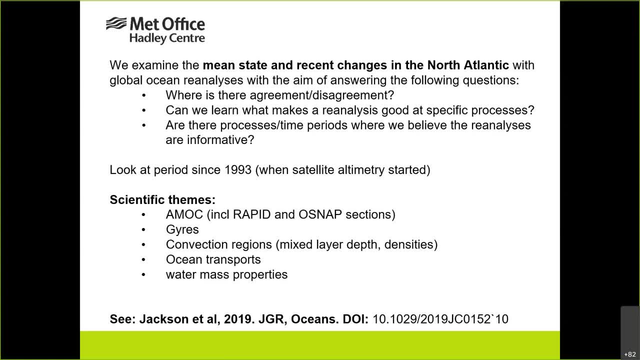 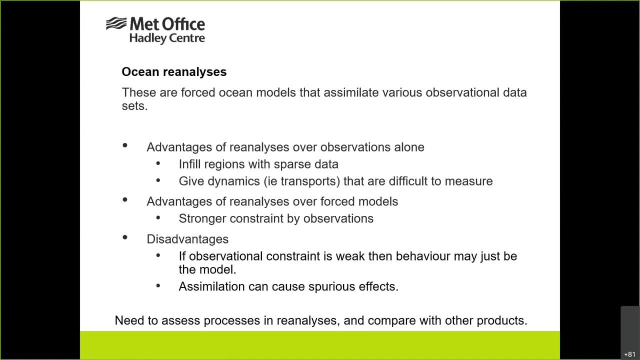 sections, Gyres, convection regions, so mixed layer densities, So I'm not showing much of that today- Ocean transports and water mass components. And at the bottom this is the reference to the paper. So, as a bit of background, what is an ocean reanalysis? So it's a forced ocean model. 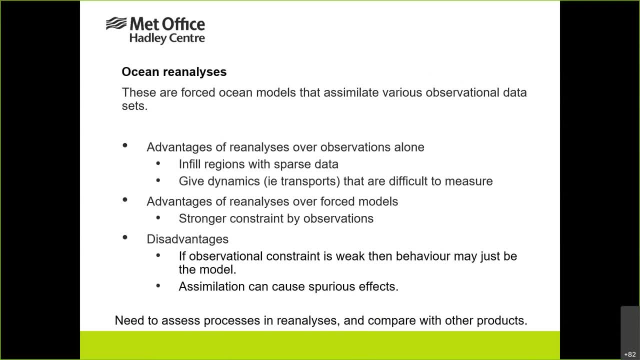 that assimilates various observational data sets. So there are advantages of reanalyses over observations alone. So they can infill regions where there's sparse data. They can give dynamic results that are difficult to measure. Advantages over forced models are basically: 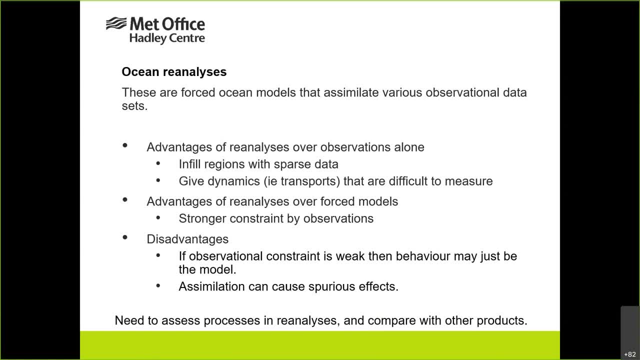 string constraints by the observations. But there are disadvantages. If the observational constraint is weak, then the behavior may just be what the model is doing. Assimilation can cause spurious effects if the model and the observations aren't in balance and you don't assimilate them. 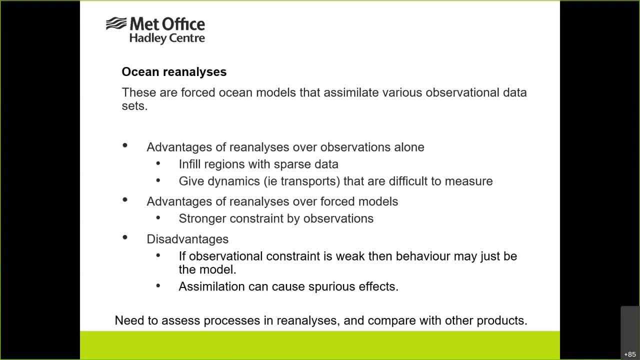 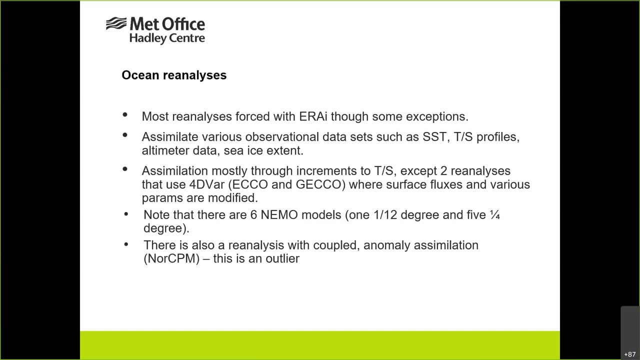 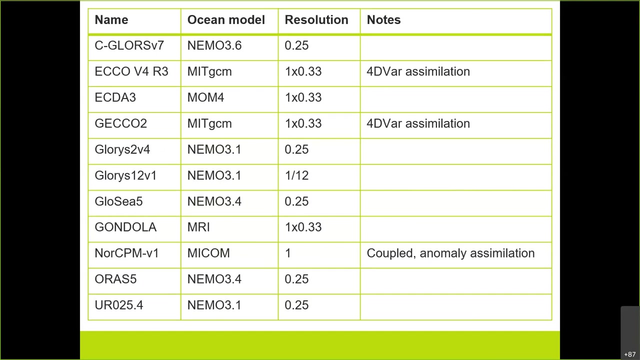 in the right way. So we need to assess the processes in reanalyses to make sure that what they're doing is, and also compare with other products. So we are using seven different reanalyses here. It's a sort of a brief table About half of our 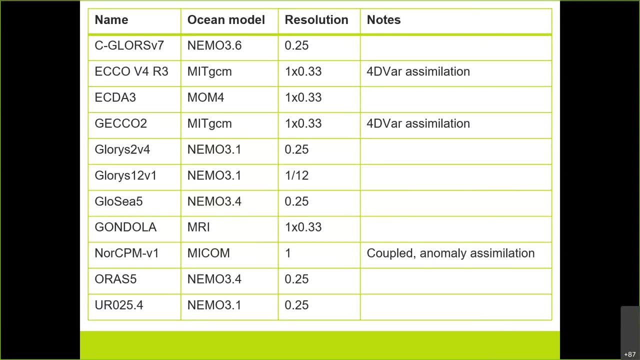 NEEMO models basically have the NEEMO ocean model And you can see that there's a wide range of different resolutions. Most NEEMO ones are quarter of a degree or there's one twelfth degree, And then the other ones are normally one degree. So most of them are forced with interim. 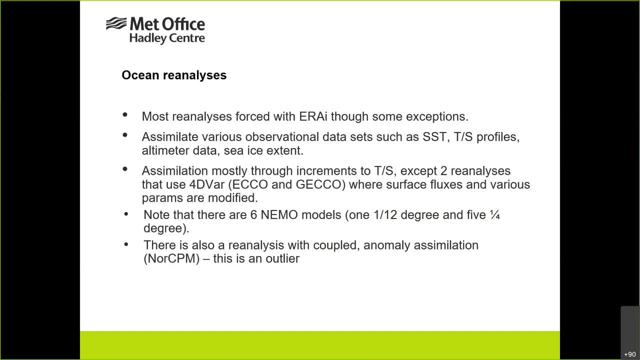 There are a few exceptions. All the reanalyses assimilate with data sets such as sea surface temperatures, temperature data, sea ice extent. They don't all assimilate all of those, all of those observations. They don't all assimilate all of those observations. They don't all assimilate all of those, all of those observations. 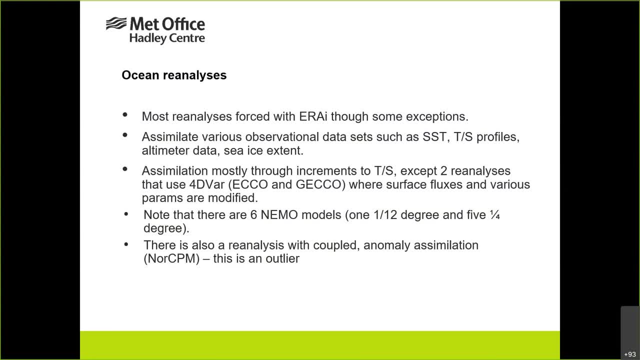 But they assimilate more of conventional types. though Ossimilation is mostly through increments for temperature and salinity, They look at where, how the the model is different from the observations and then you can apply increments towards them. viewers use 4D-VaL, which uses a very different assimilation method, where, instead of using increments to 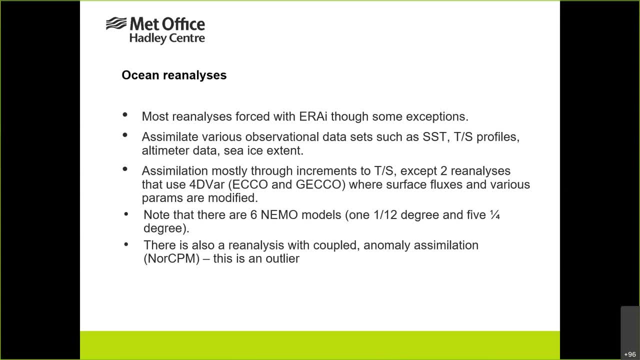 temperature and salinity. you modify surface fluxes and parameters, for example golden mixing, to essentially try and achieve better temperature and salinities in comparison with the observations. So, as I said before, there's six NEEMO models, one of which is called Pelford Green. 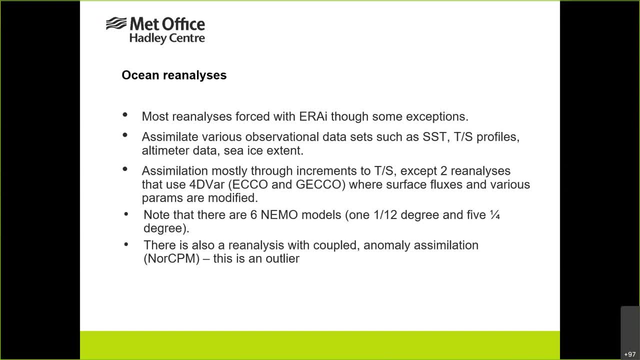 There's also one reanalysis which is an outlier, and that's NOR-CPM. It's partly an outlier, but it is coupled, although it is a reanalysis. So, yes, it basically coupled an atmosphere and ocean analysis together, but maybe more so in that it only assimilates anomalies. 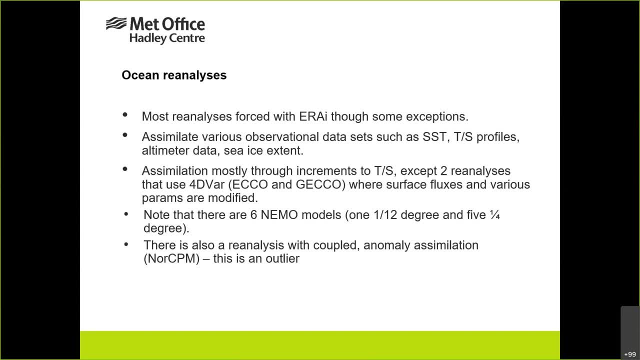 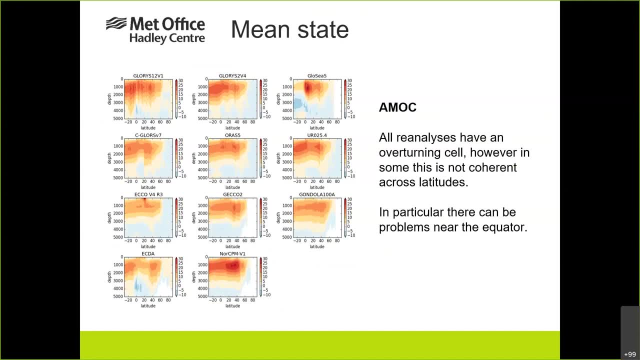 so it doesn't try to constrain the mean state. So look at some results, Looking at the AMOC, looking at the mean state of the AMOC. so all the analyses have an overturning cell. however, in some this isn't coherent. 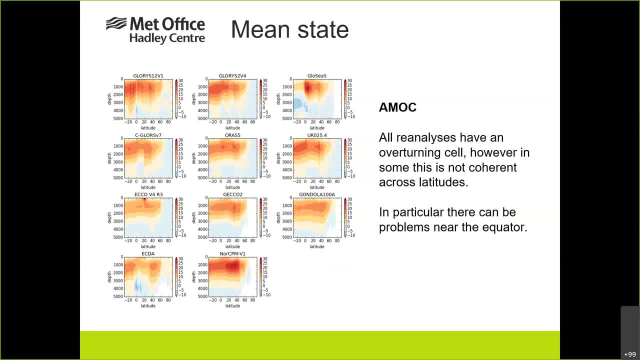 So generally they seem to be pretty coherent in, say, the subpolar gyre, but less so further south, particularly if you look at Glossy 5 here, which is our reanalysis. It's fine north of 20 north, but near the equator there's these large values and then it's two. 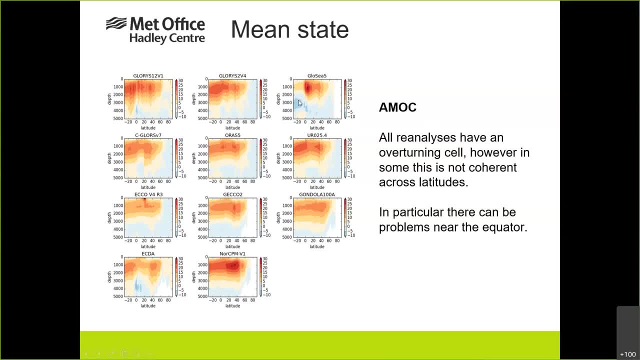 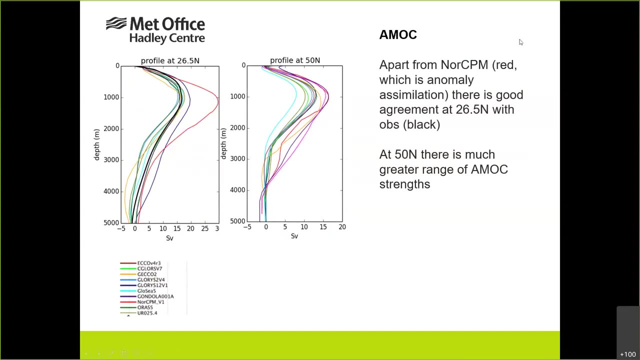 weak in the South Atlantic And we believe we know why that is and that's the way we're doing the assimilation. that's been corrected for future, hopefully. If we look at 26.5 north, we can compare the AMOC profiles with RAPID. That's what we're doing on the left-hand plot here. 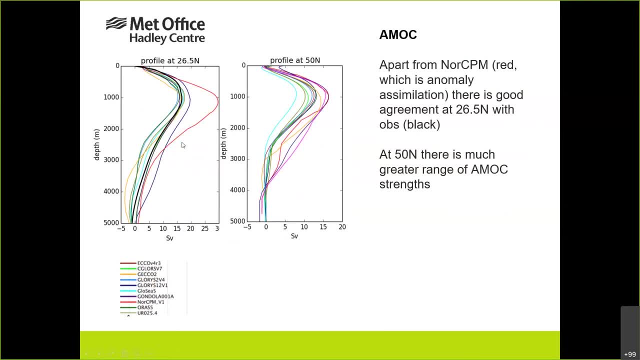 If you ignore the red one here which is the NOR-CPM, which isn't constraining the mean state. they all do pretty well at getting the magnitude of the AMOC and some even manage to get pretty well the depth profile. 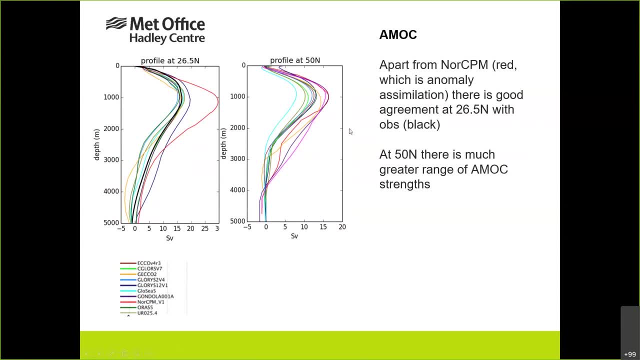 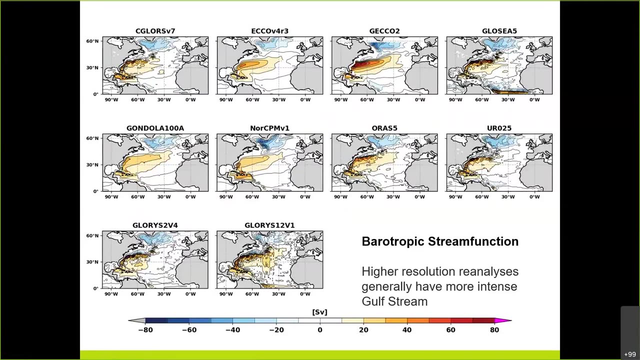 If you look at 50 north, however, there's a much greater range of AMOC strengths and a much greater range of depths as well. Looking at the bell-top extreme function, it's just shown here. So the main thing to see from this you can see if you look at the. 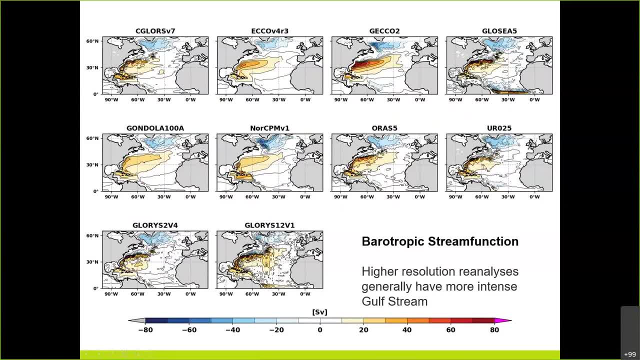 subtropical gyres. rather, a number of these have very intense gyres near the western boundary. This is because they have intense gulf stream And these are all the higher resolution models, and so they have more intense gulf stream and much more eddying. 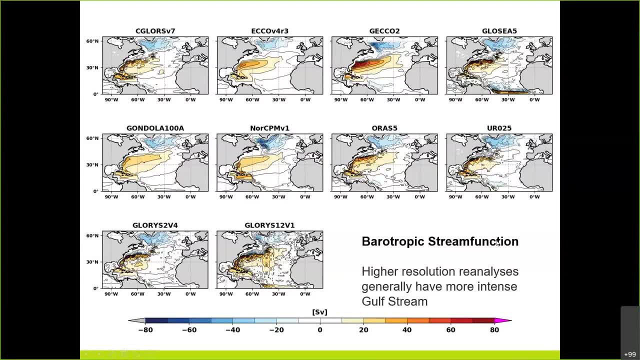 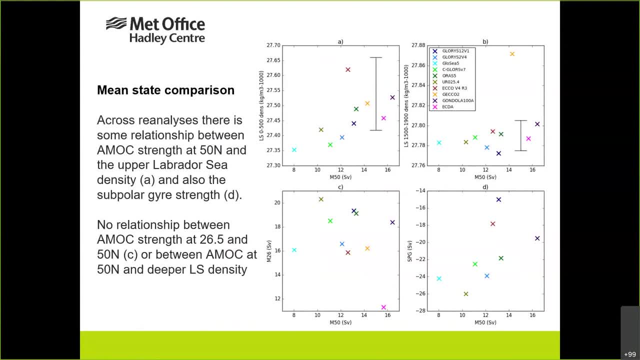 And as the red gruppe goes over here, reversing towards a point where we can see much more light, center and value, but actually So when we display this particular data- tooopφere tograd microgravity- you can see that on the upper left-hand. 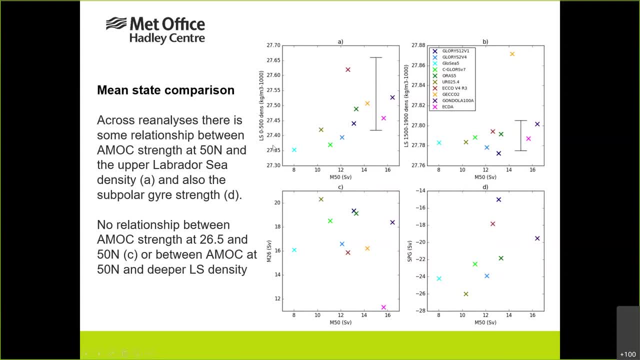 here theoue terminal times of Redmond Tri många also down, easier to obtain żeby bridge gulf. lesser level of anлатiesch And if we compare this to the Left 하 Humor Swedish by Look Down to ASH Pilots. there's an information. So we can look across these analyses. I'm sure many of you know that in many studies the AMOC is related to the density in the Labrador Sea example. so it's what this top-left section count is, showing Comparison with the AMOC strength: 50 north T islands and low density density in the North and Westltry geami. 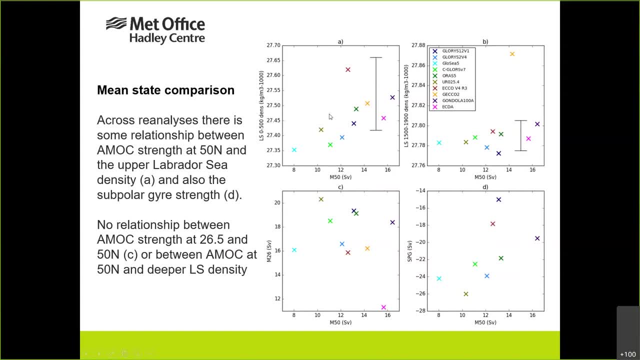 in the 0 to 500 meter range and you can see that there's a significant correlation there. so, um, renalcies with a- it's a more dense- have a stronger aim up. um, however, um, you have two observational estimates which give this big bar here. um, so it's quite difficult. 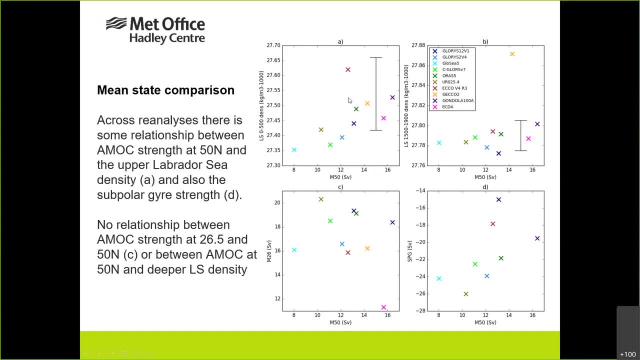 to use the observations to say how, how strong from this um, this relationship, you might think the um. there's also a significant relationship if you look at the aim, compared to the subpolar jar strength. so renalcies with a stronger amok have a weaker subpolar jar strength and that's. 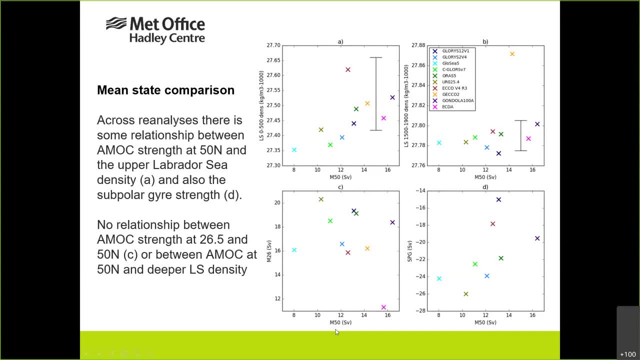 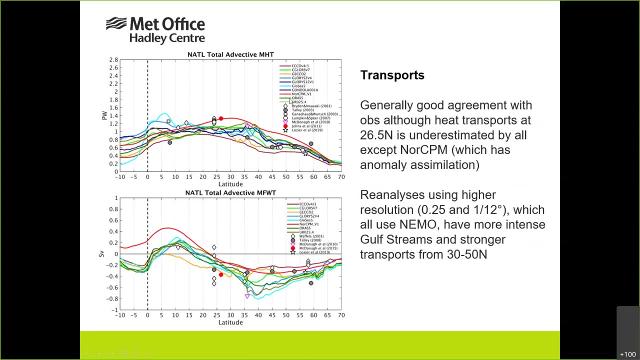 a significant correlation um comparing the amok of 50 and 26 north. however, there's no significant relationship there. so if we look at transports um again, you might want to ignore the norwegian one, which isn't um constraining the mean state um there's. there's two things to um pick out from this. so the top one is the heat transports the. 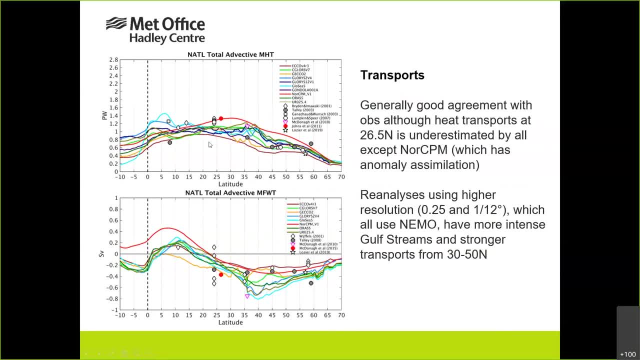 bottom one is the freshwater transports. so if you look at around um 26 north, there's a number of different observations there, that's those that have been shown in the symbol um, and you can see that all the apart from the north cpm um, all the renalcies are undervalued um. so you can see that. 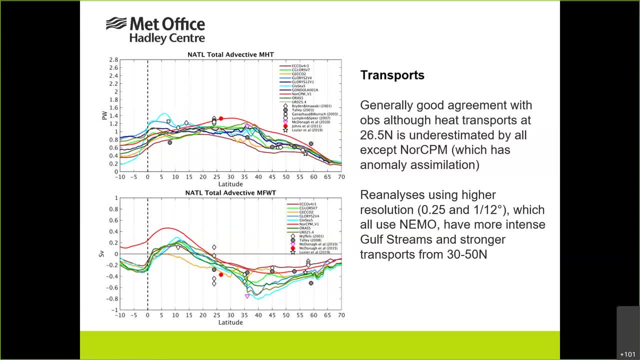 we're estimating the transport there um. one other um aspect to point out is that if you look at 40 north um, all the reanalyses, all the renalcies which are sort of bluey green colors, so there's suppose all the um, all the rest, all the renalcies that she used nemo, so they have stronger heat. 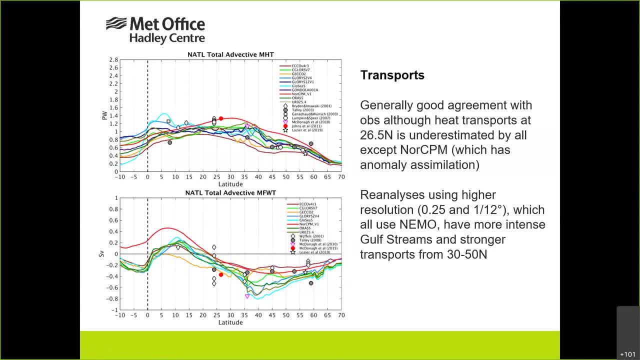 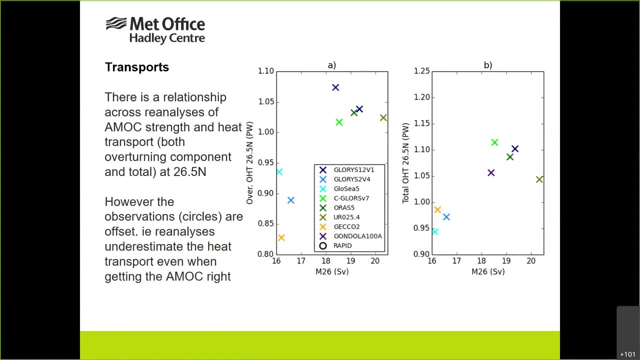 transports and fresh trans fresh water transports around 14 or um and they also, you know, they're also having a higher resolution and a more intense gulf stream and we think it's that this more intense gulf stream is giving greater transports at this latitude. so we can look at particularly 26 north um, many studies and the observations as 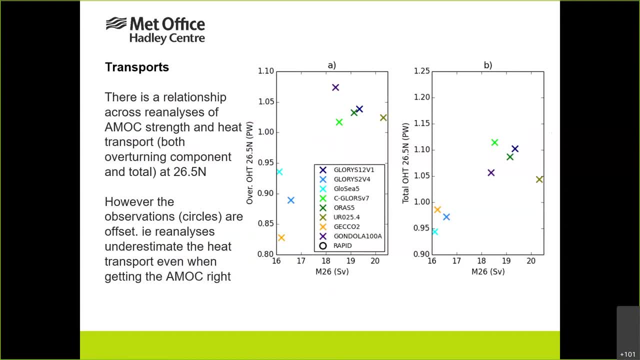 well show relationships between the um, the aml 26 north and the heat transport and you can see there's a good correlations across across the the ensemble And this is, yeah, overturning and the total heat transport. But if you add the observations which are these circles here, you can see that offset from that relationship. 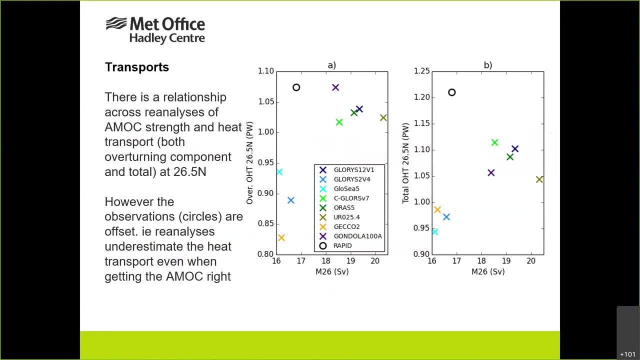 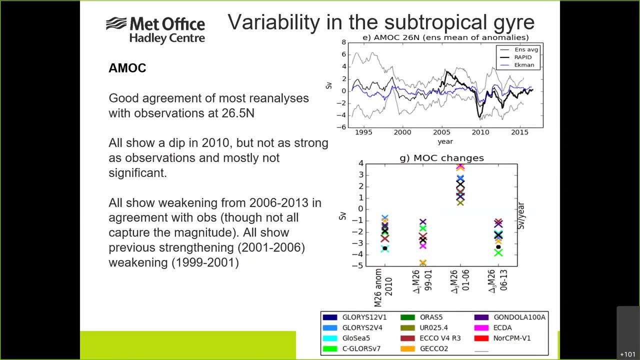 So it's saying that the reanalyses are underestimating the heat transport, even when they get the aim off right, And this is something that's also seen in forced and coupled modes, this similar sort of bias. So moving on to variability, starting from the subtropical gyre. So that's. 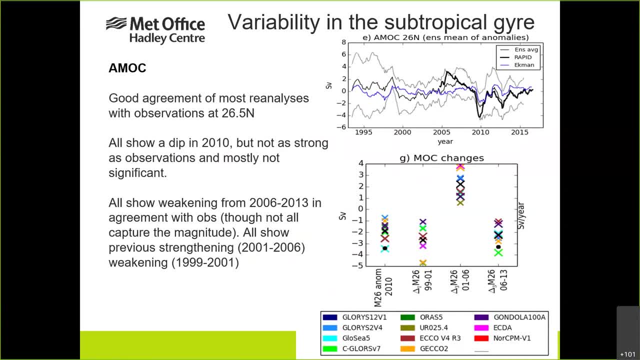 25 to 45 naut. So, starting from looking at the aim up at 26.5 naut- And I'm just looking at the anomalies of the time series And I've got the ensemble mean spread in the black and grey lines here of 25 to 45 naut- 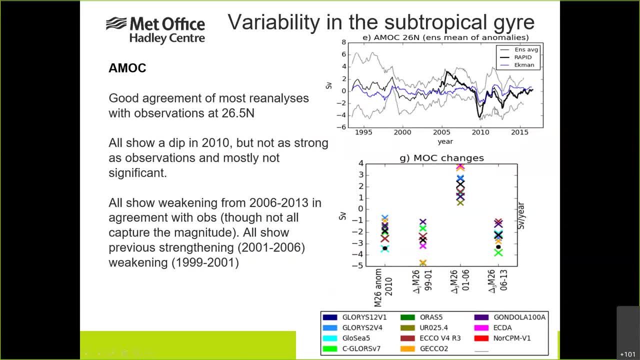 And then the thick black line is showing the rapid observations And you can see quite good agreement with the ensemble mean. in terms of the variability, You can see a sort of a weakening from around 2006,. get a stronger weakening in 2010, and then the sort of internal 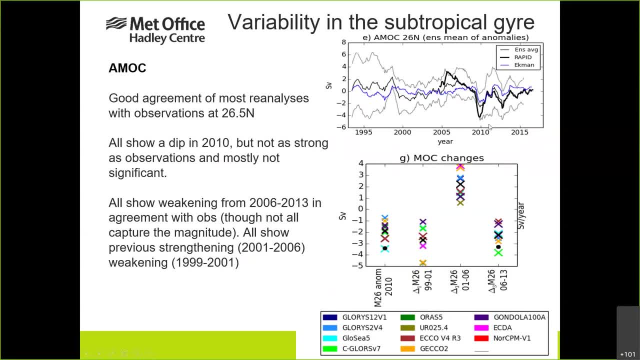 variability after that. But you do see this, it's not getting all of that dip in 2010.. And actually, if you look at the Ekman, which is the blue line, it seems to be mainly just getting the Ekman. However, that's not true necessarily for the individual reanalyses. 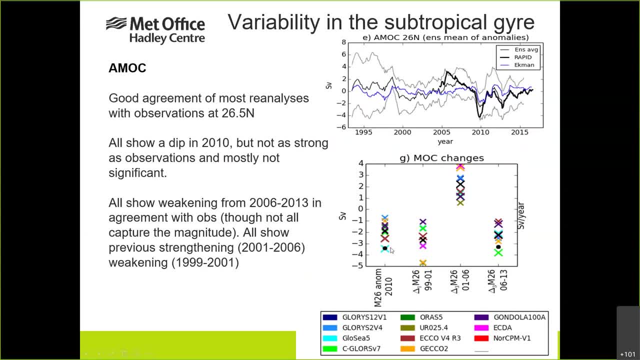 So bottom plot in the left hand column that's showing the aim op anomalies in 2010.. For all the different reanalyses and the big crosses are where that's statistically significant in the time series. So all the reanalyses are showing a dip in 2010,, but most of those are not showing as 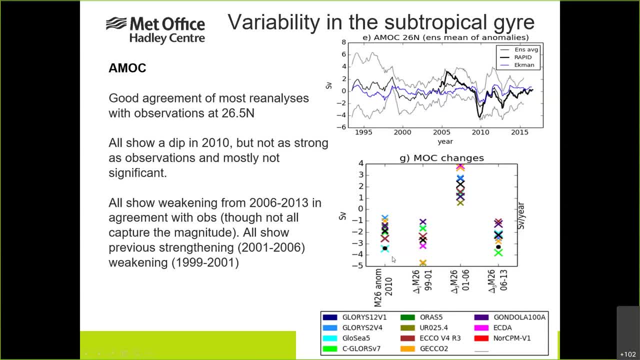 strong a dip as the observations which are the black dot. So we can also look at the other feature of the rapid observations. this is weakening in 2006 and 2013.. And if you look at the different reanalyses, most of them actually show that's a significant 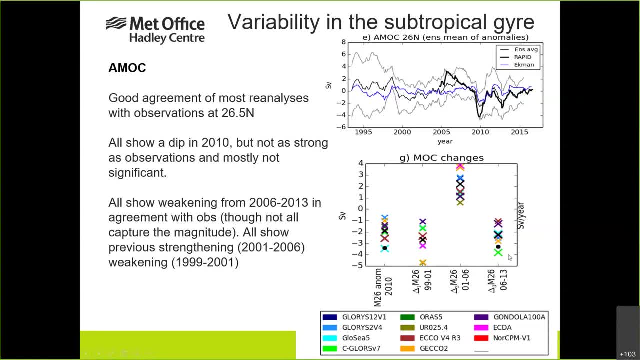 weakening over that period, though in many it's not as strong as the observations which are again in the black dot. So we can then look prior to the observation starting. what do the reanalyses suggest? So it will seem to suggest that in 2001 that there was a weakening. so we all seem to get after 2001-2006 a strengthening. 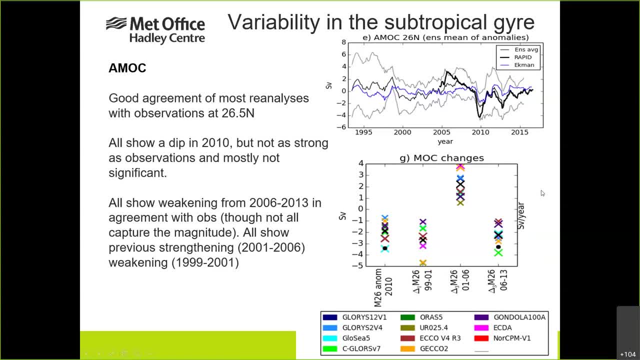 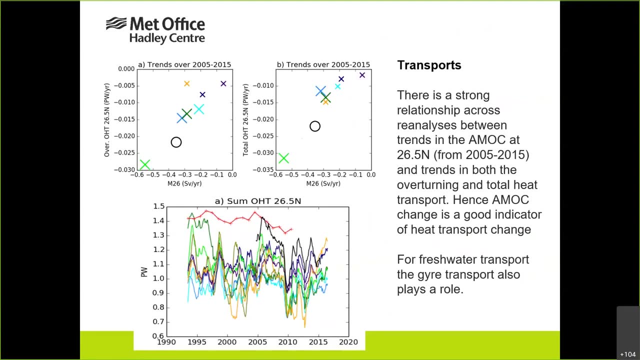 of the AMOC. So this does seem to show some evidence for multi-annual decadal variability of the AMOC. So these changes in the AMOC at 26 North, These are unsurprisingly seen in the transports of heat. so these time series, here you can. 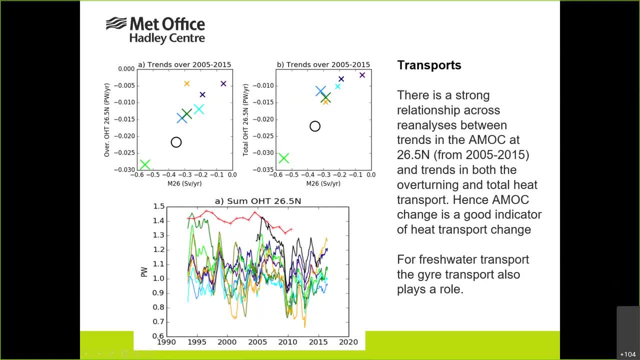 see that the weakening and the big dip in 2010,. this weakening trend is strongly related to the trend in the AMOC and you can see that across the different reanalyses and this relationship seems to agree with the relationship in the observations as well. 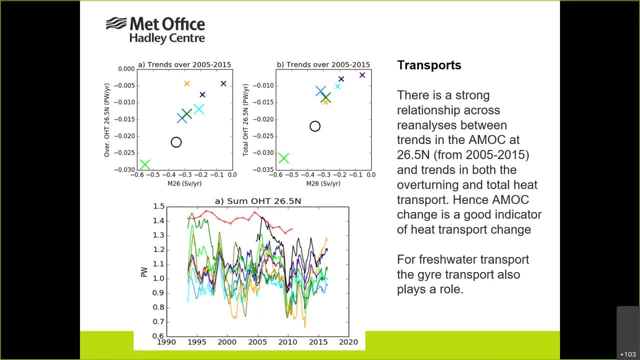 The first thing I'd like to say is that I think it's important to note that this is not the first time that we've seen this. It's not the first time that we've seen this. It's not the first time that we've seen this. 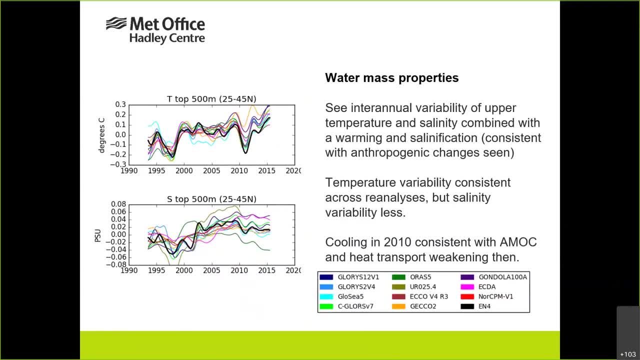 It's not the first time that we've seen this. So if we look at the temperatures and salinities in the subtropical gyre regions, that's 25 to 45 North, we see the gradual warming and salinification of the gyre, as well as some. 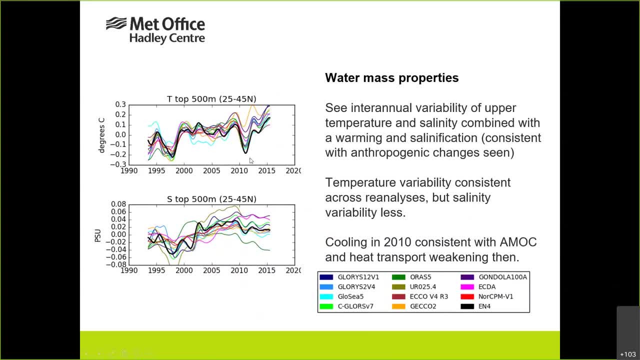 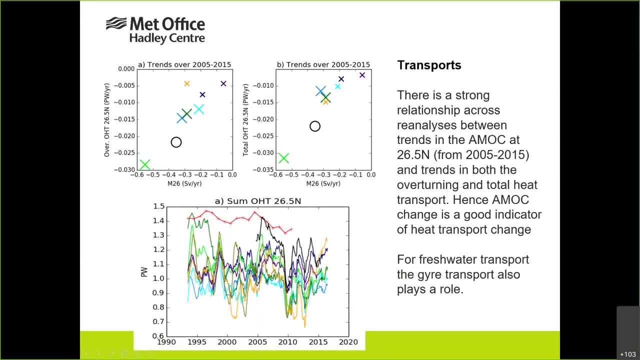 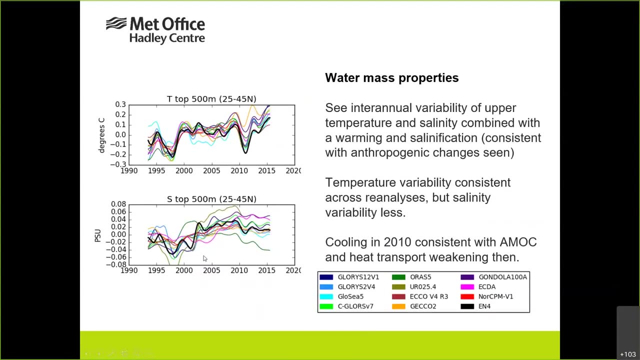 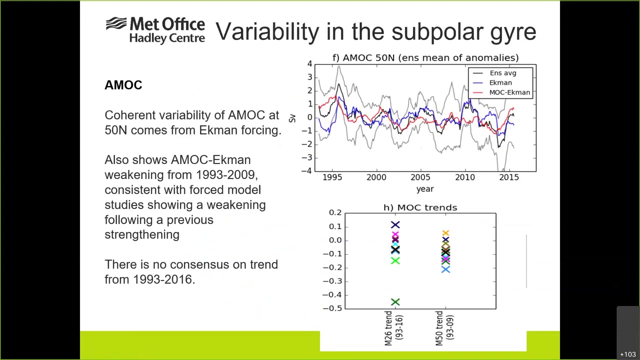 inter-annual variability. In particular, you can see this big dip after 2010,, which is believed to be related to this very weak heat, And you also notice that the salinity is much less constrained than the temperatures. That's the subtropical gyre. we now can move on to the subtolar gyre. 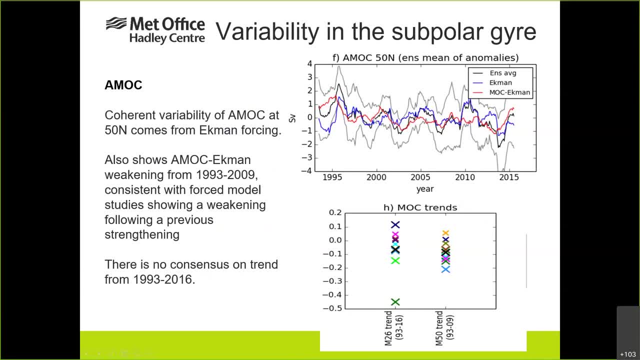 AMOC anomalies here show a quite consistent inter-annual, multi-annual variability. If you plot the Ekman- that's the blue line over the top- you can see that corresponds very well with those inter-annual changes. So that's obviously a key component of the variability. 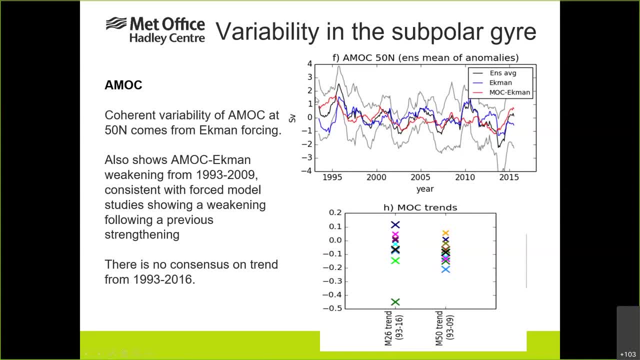 If you subtract the Ekman from the Ensembl average, that's the red line, and so now you see the Ensembl is over this time period. This is consistent with other studies, particularly using force models, Which showed the AMOC strengthening up to mid-90s and then weakening over the period. 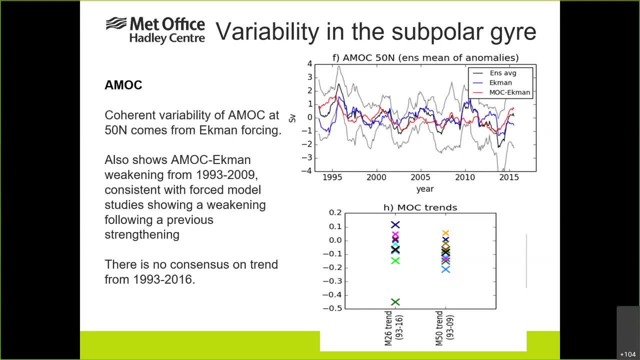 to 2009-10. And this is believed to be called changes in the NAO. So we can look now at all the individual re-analyses in the same way. we've got the trends from 1993 to 2009.. 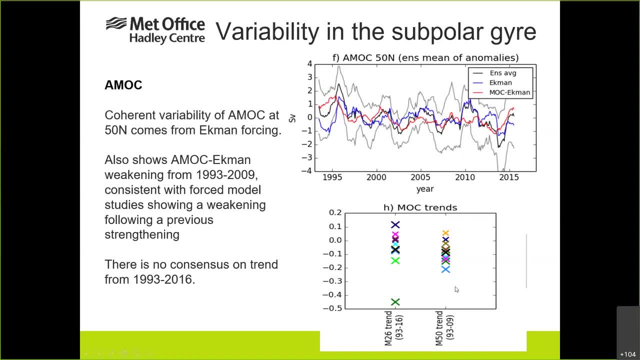 In all the different trends. So we can look now at all the individual re-analyses in the same way. We've got the trends from 1993 to 2009.. In all the different re-analyses, most of them, most of the re-analyses- are showing: 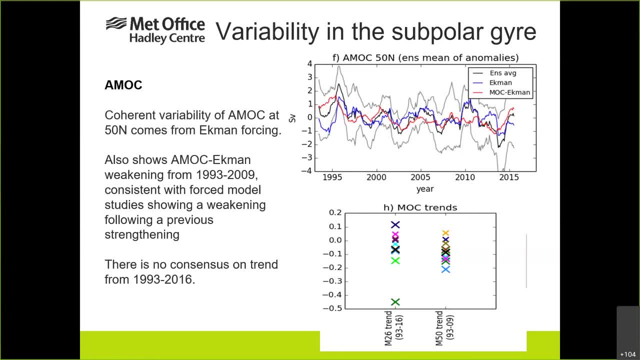 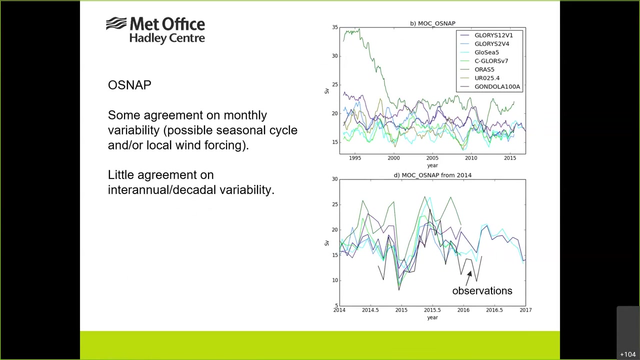 a significant weakening trend. Though a few are not showing significant trend, most of them are showing significant weakening trend Over the whole time period of this to 2016,. there's no consensus on the trend. no trend at that point. We did look briefly at the OSNAP section in a few slides. 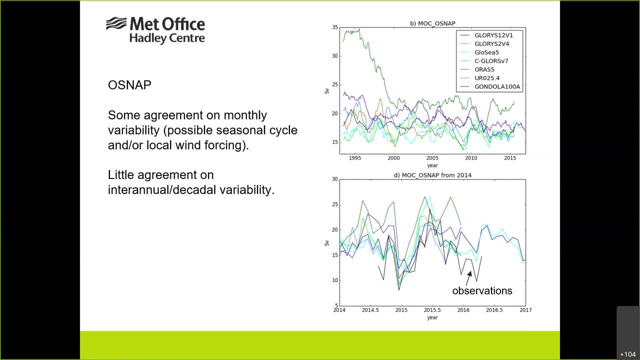 The OSNAP section is around 55 more and measures the AMOC in density space. it's been going for well. we've got observations here anyway for the paper for about two years. That's showing this black line here. 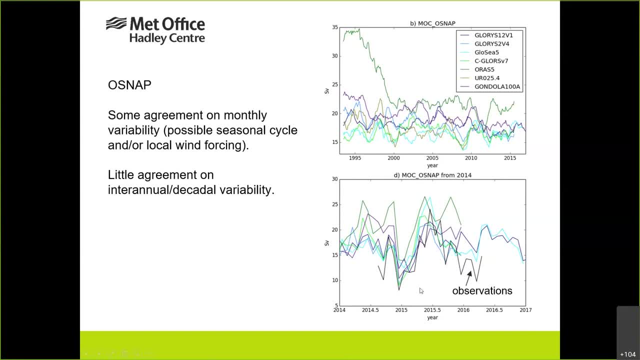 These are monthly values, So you can see the analysis actually do a surprisingly good job at picking this dip at the end of 2014.. And then starting in 2016.. And then strengthening and then weakening again. We think this is possibly partly the seasonal cycle and or local wind forcing, which is 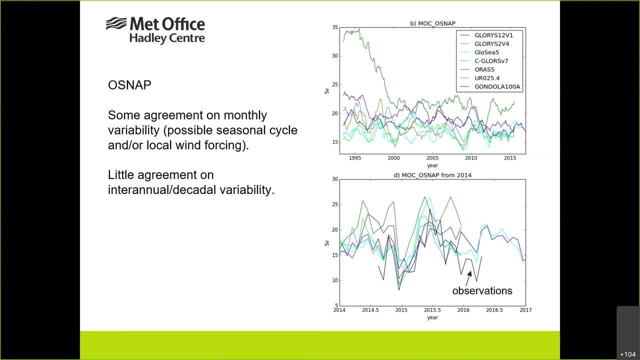 why all the re-analyses get that. quite well, If you look at the inter-annual decadal variability, which is the top plot, actually there's quite a lot of quite a lot of difference on that, so there's little agreement. 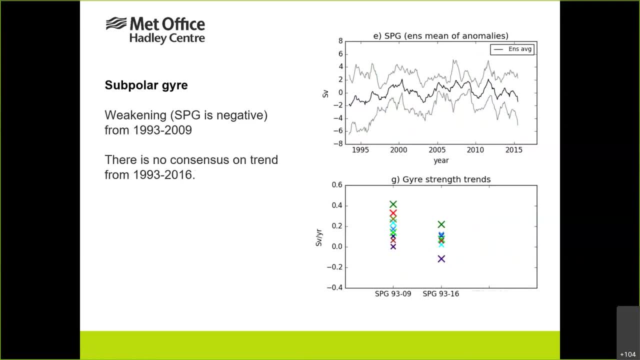 So then, moving on to the gyre, so the subpolar gyre is negative. So when we see this sort of positive trend in the ensemble, that's basically a weakening. And if you look at, yeah, from 2003 to 2009,, you can see that most of them are showing. 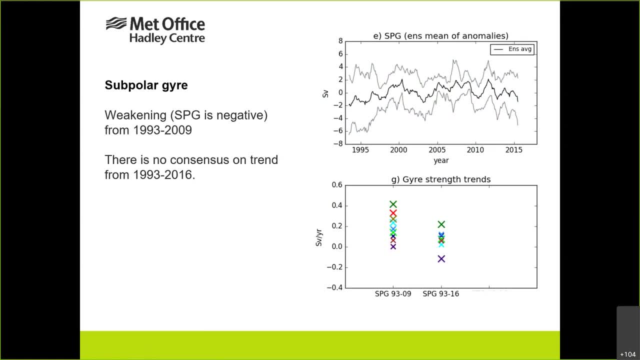 a significant weakening of the gyre, Which is again in agreement with other other studies and observations. But then if you look at the whole time period from 2003 to 2016, actually there's there's no significant, no consensus on trend in that time period. 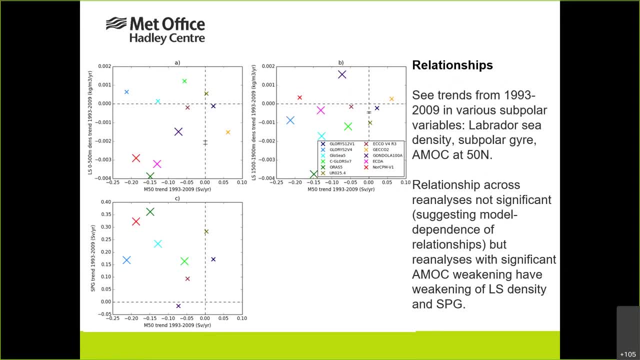 So we've got a number of different quantities. in the subpolar gyre we see trends from over the 93 to 2009 period. So there's the Labrador Sea Dental, There's the Labrador density, which I haven't shown, There's also the subpolar gyre and the AML 50 North. 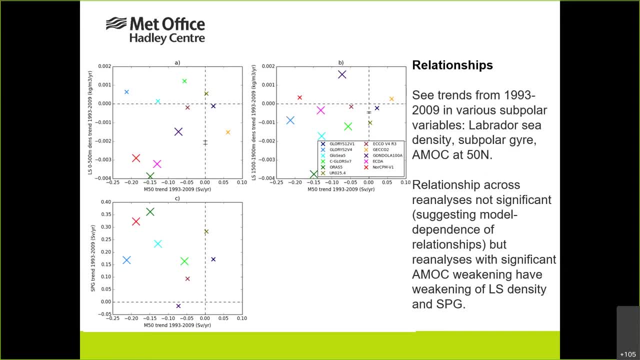 So we can ask: are these, are these trends related in any way across the ensemble? And the answer to that is basically no. So many of the reanalyses have significant trends in these quantities, but but those relationships are different between the different reanalyses. 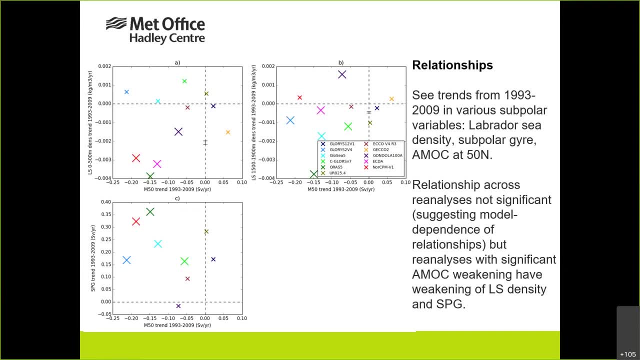 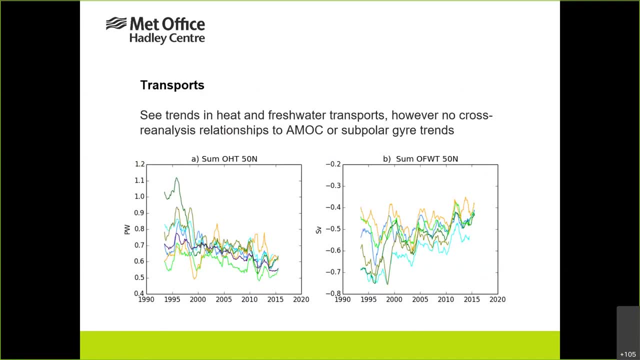 So yeah, which suggests that there's a model dependence of the relationship. So we can also then look at the heat and fresh water transports that 50 North and, like the AML and the subpolar gyre- these are both. these are all showing quite strong trends. 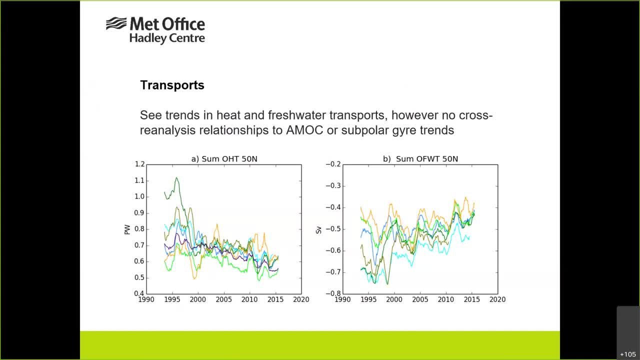 weakening trends as well. However, when we did similar scatter plots comparing the trends in the in the transatlantic transports to the trends in the AML and the subpolar gyre, we didn't see any relationships there, And that's possibly because the way they're interacting is different in different reanalyses. 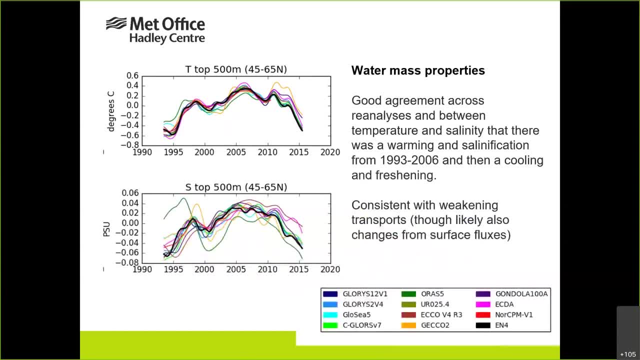 So then, finally, looking at the water mass properties, the temperatures and salinities in the subpolar, the upper subpolar gyre, unlike the tropical gyre, it's much more vertical. So if we look at the 53 C, then we see there's a significant increase in tall rigidity. 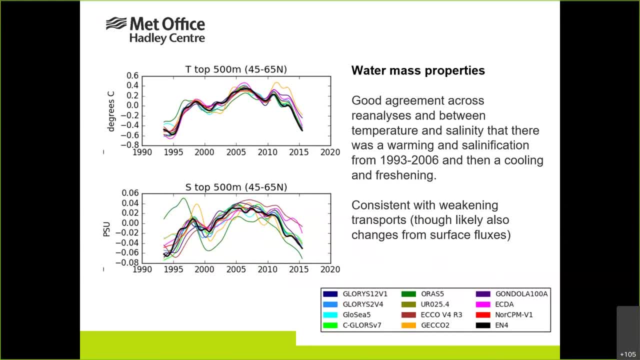 in the subpolar gyre with the fine and hollowimen and the large sludge, And we also see that, as you can see, there's a decrease in the water mass property. Think about the structure of the region of the subpolar gyre. you can see that against. 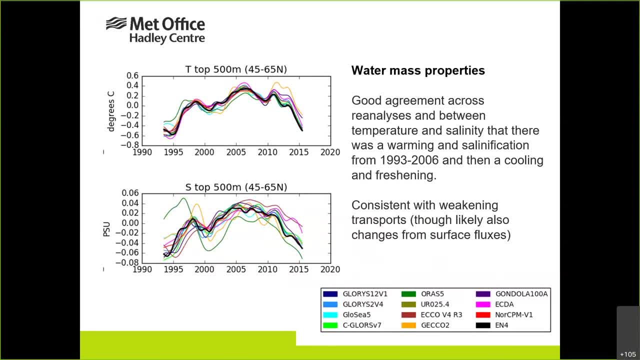 the mutual, The, the. the area of the subpolar gyre is much more hidden, So at the bottom of the slide you can see the higher and lower, the lower, the lower transatlantic and the lower transatlantic, and the lower transatlantic and the lower. 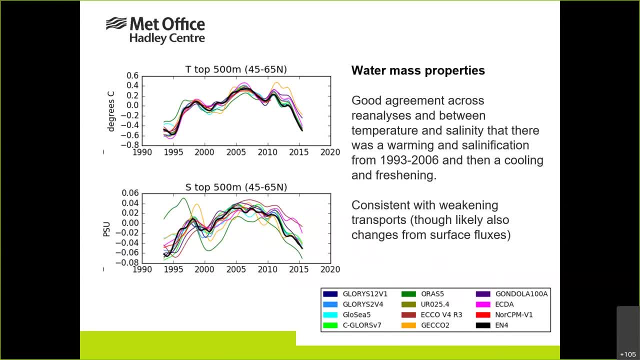 transatlantic. So this is, this is a condition for that- that as well, we can look at different temperatures. So it is important to note that there have been changes from surface fluxes, which may well have also had an impact. 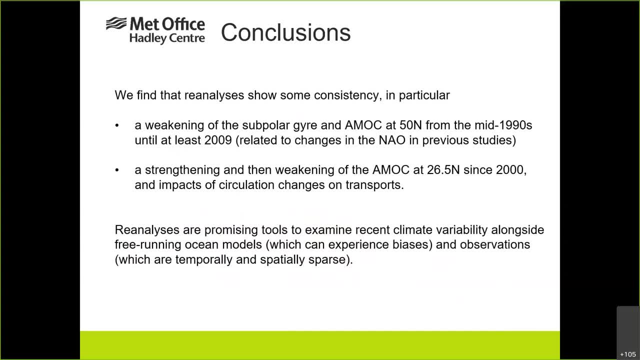 So conclusions? So we find that the analysis shows some consistency. In particular, we see a weakening of the subpolar gel on the A0 from the mid-90s to at least 2009.. And we should note that in previous studies this has been related to changes in the NAO. 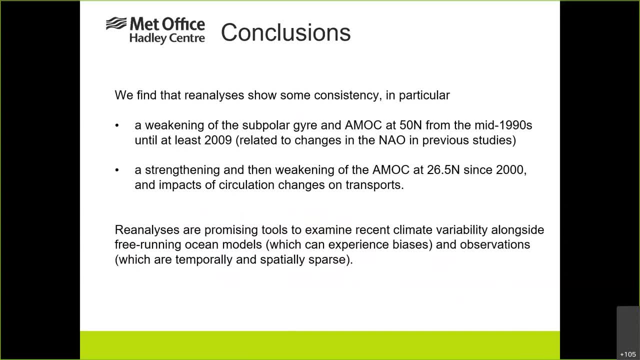 A strengthening and then weakening of the ALOF at 26 NAO since 2000, and we've seen impacts of this separation, changes on the transports And I should say in conclusion: so the analyses are promising tools to examine the recent climate variability, alongside free-running ocean models, which can experience biases, and the observations which are temporally and spatially sparse. 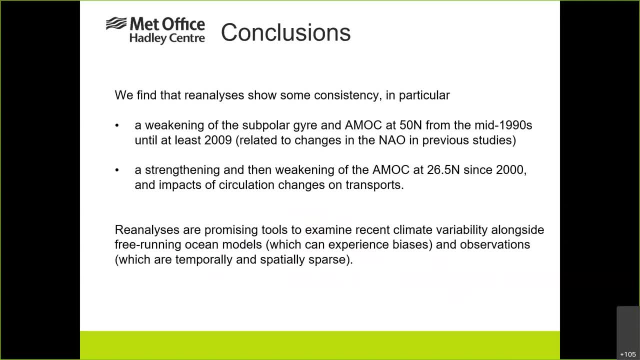 Thank you. Thank you, Laura. So if you have any questions for her, use the raise your hand button or you can type your question into the chat box. I see one question from. I don't see your name fully on there, but if you can unmute yourself, go ahead and ask your question. 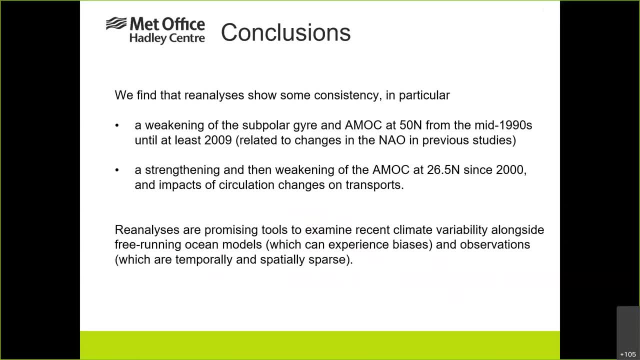 Okay, Is it on here, Laura? that's very nice stuff. My question is, although in this paper you focus on real analysis, I'm just wondering the relationship between 26 degree north and 50 degree north of the AMOC for the free-run four-way carbon model. do we see any relationship, or it seems as if it doesn't have any consistency or coherence? 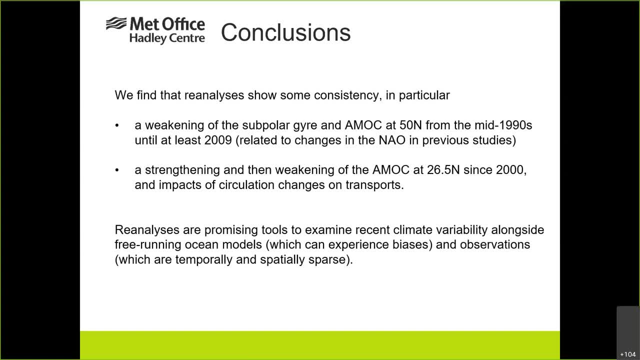 Do we see any relationship, or it seems as if it doesn't have any consistency or coherence. I'm sorry, I think I have a question. I'm sorry, I think I have a question. The sound quality was. I couldn't really make out what you were saying. the sound quality was quite bad. 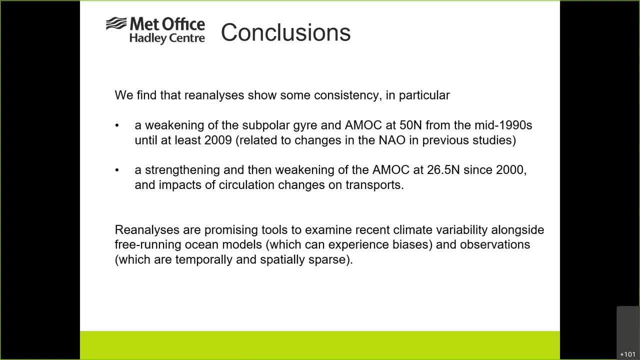 I think you said the relationships between the AMOC at 26 and 50 north. is that right? That's right. yes, I'm wondering for the carbon model whether they have any relationship. I think it's difficult to tell in these reanalyses. 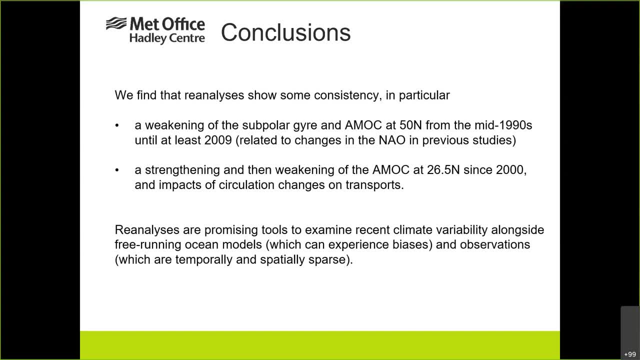 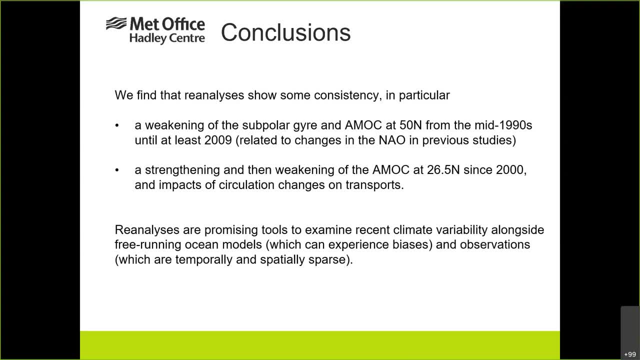 Within an individual reanalysis, you might expect there to be some relationship, for example, to: However, we don't have long enough. I mean, the runs are only- I think it's 24 to 5 years, so it's not really long enough to see that. 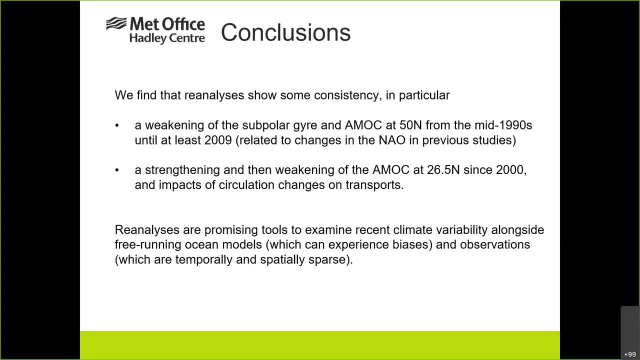 So we don't have long enough. I mean, the runs are only, I think it's 24 to 5 years, so it's not really long enough to see that. Okay, thank you. Okay, thank you. Another question. your name appears as W Large. 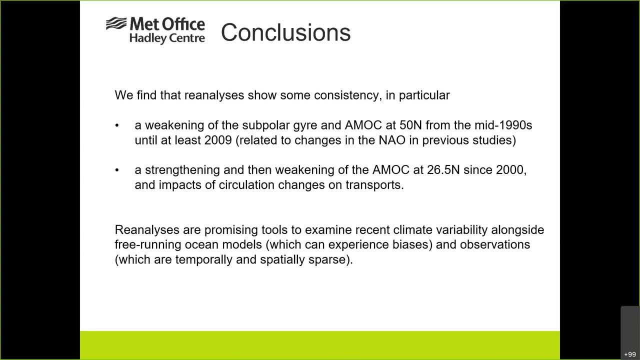 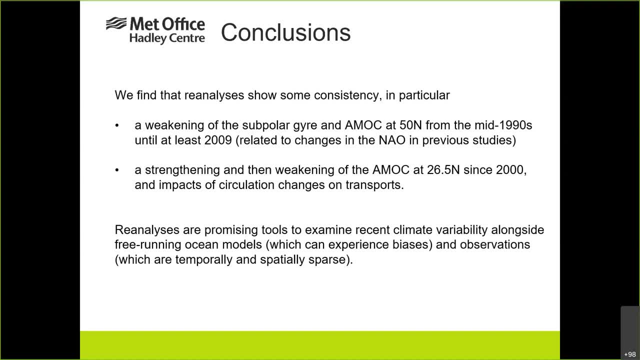 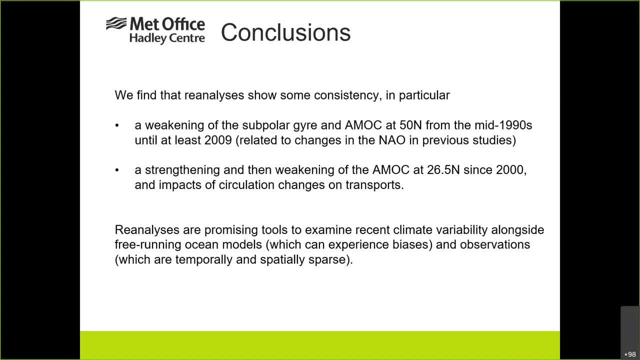 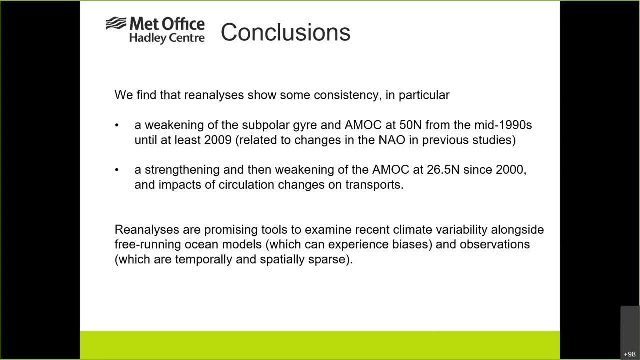 I mean, they're giving very different answers in some places, and that seems to have been the case for many years now, and yet they're the best each group can can come up with what. what do you really think is the underlying reason for the difference from one reanalysis to the other? and when you look at the 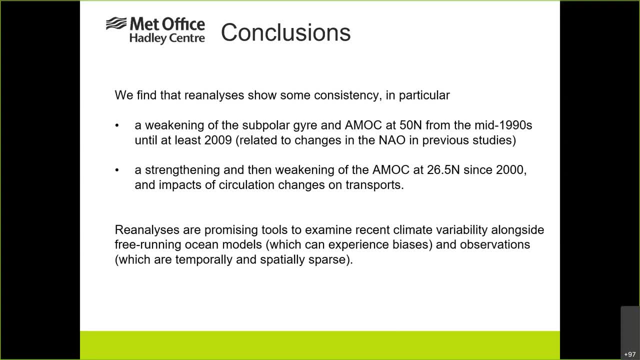 fields? uh, it's always there. so do you have any thoughts on what is fundamentally causing that spread? that's a very difficult question. i don't think i can. um, i mean, i guess i mean with a reanalysis you've got to balance, you know, i guess you only take an ideal reanalysis you have to have. 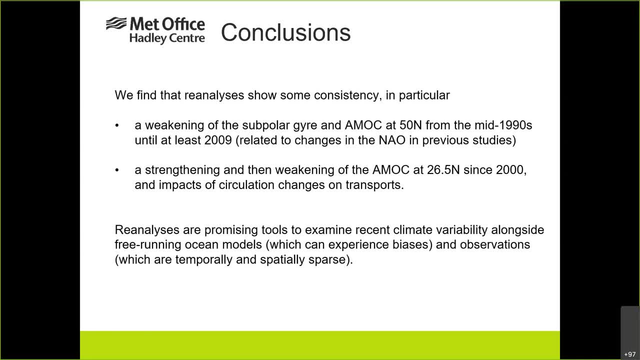 an ideal model, an ideal assimilation system and preferably, ideal observations, um, and i guess everyone comes at it from slightly different angles- um, in terms of development, and maybe what, what their, what their priorities are in terms of improving. so maybe, maybe that's what it is, but yeah, i, i can't say, i'm afraid. 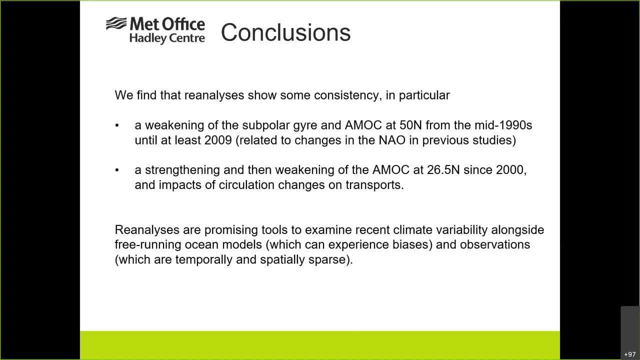 okay, okay, okay, we have a couple questions in the chat box. uh, we have one comment from tony rosati says: don't you think a non-stationary observing system makes it difficult to look at trends, particularly with argo starting in 2003? yeah, this is definitely true and that is definitely a caveat. um on on. 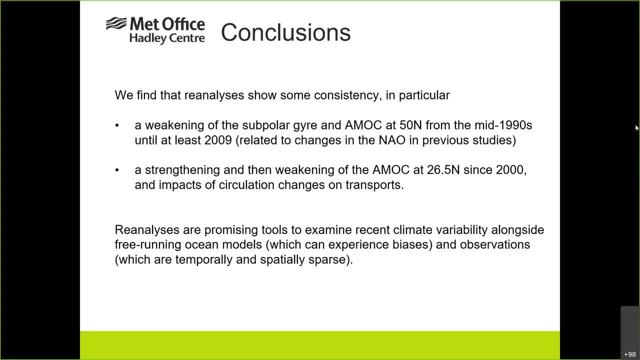 these, or particularly on the trends, um, it's so certainly one reanalysis there there's. there's a very clear change in what happens as the up, as we reannounce, as the observational system changes. It's not so obvious in others. I mean, I agree it's a question and I guess the way to answer it is to perform some experiments where you take out some observations and see what happens. 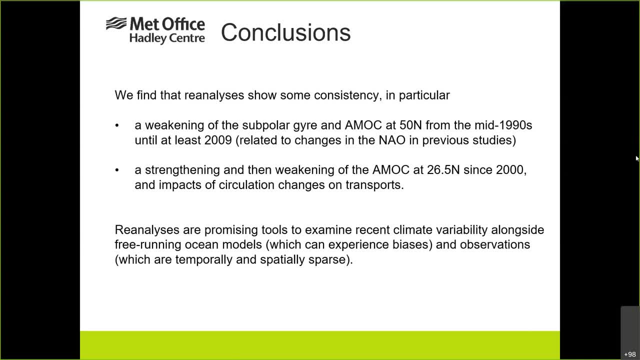 But I mean, I guess the fact that the general picture agrees with, say, force models and other things is certainly encouraging. Can I make a comment? Yeah, I just want to actually comment. This is the same topic with the bill bill largest comment: that. 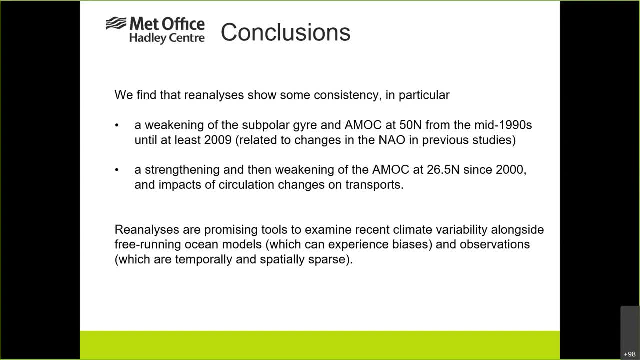 We have spread, but the spread diminishes quite a bit. Once the Argo, during the Argo period, Yeah, constrained, constrained the system better because we didn't have Such as sparse data Set then then then the reanalysis come much closer together. 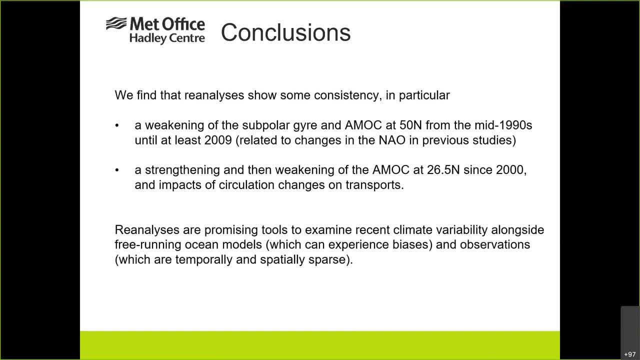 Yeah, I mean yes when we start the session. I think it does depend on what you look at, as you say. I mean certainly if you look at some deep properties, the Argo, I imagine it makes a huge difference. if you look at heat content, for example, it makes a big difference, I think, in terms of the constraining. 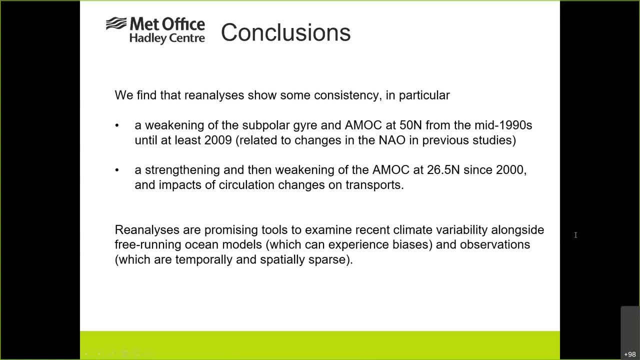 Okay, we have a question from Sergei. He asks first, says thank you for the presentation. Let me scroll back up. What do you think? What do you think are the ways of which you think reanalysis should improve, given the available observational data? 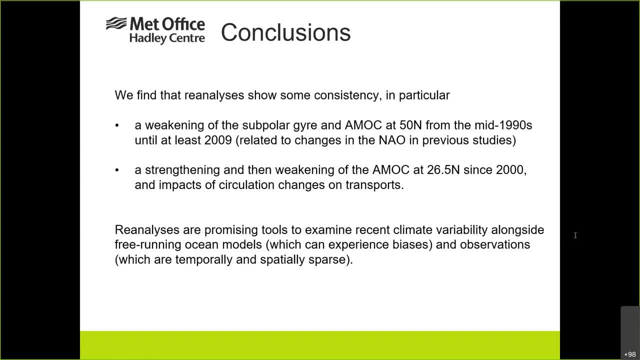 Again, another good question. so I'm not- I'm not somebody who runs reanalysis, So It may be better to ask somebody else This question. I mean, I think I think making sure that you, you Test, a lot of reanalyses are developed for particular purposes, like for initializing models. 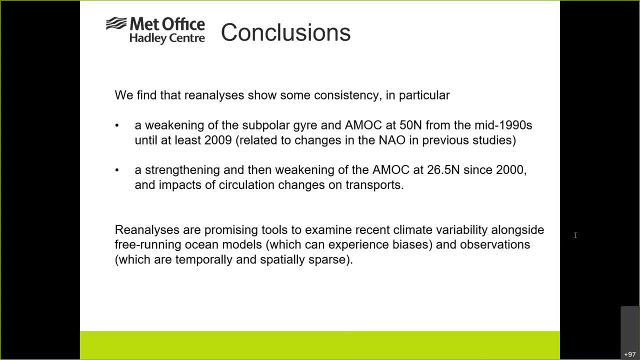 Finish initializing, say, coupled models Or for sort of seasonal forecasts and that sort of thing. And so I think, maybe taking a broader look and seeing how different processes work in your reanalysis- and Sometimes you come across things which make it clear, like for us that when we plotted the AMOC full stream function, we could see that there was something going on with the equator. 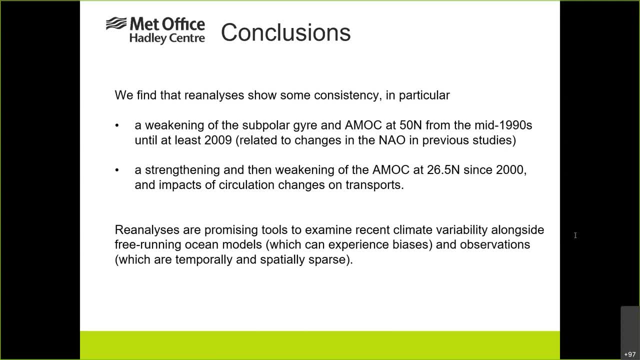 Which we needed to sort out, but in general I don't know is the answer Okay. another question: I'm sorry If I Sorry if I mispronounce your name question from. is it Devin Narayana Rao? yes, 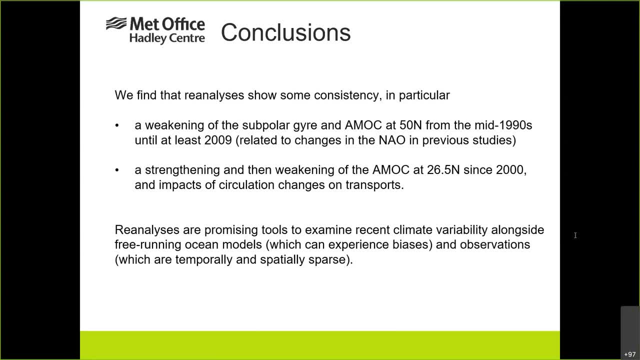 Are these reanalysis open access, publicly available? I know echo and or a 5 are open access. Okay, so the the data from our paper is. there's a link for paper to Website where you can download, but that's only these, the time series and things plotted here. 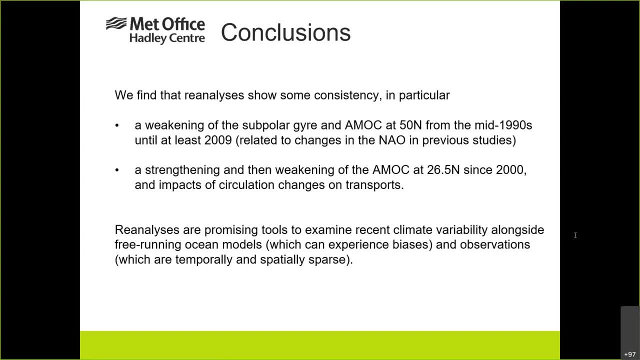 So a number of the Nemo Reanalysis are part of the Copernicus Marine services and the data is available to download From them. I don't and I don't know about All of them or the other analyses, but yeah, so obviously I can. 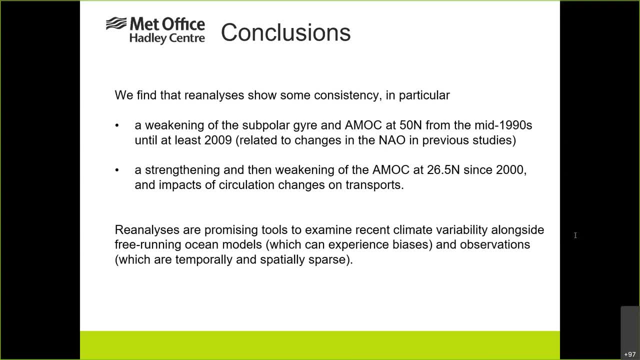 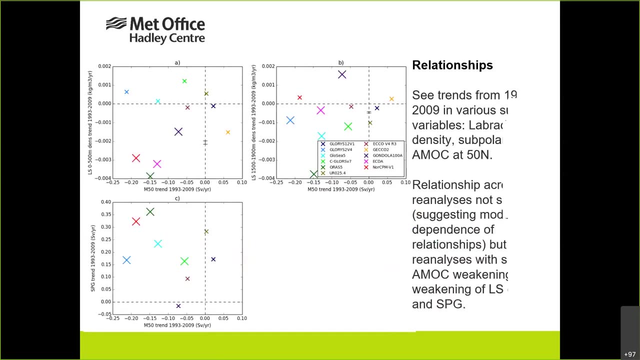 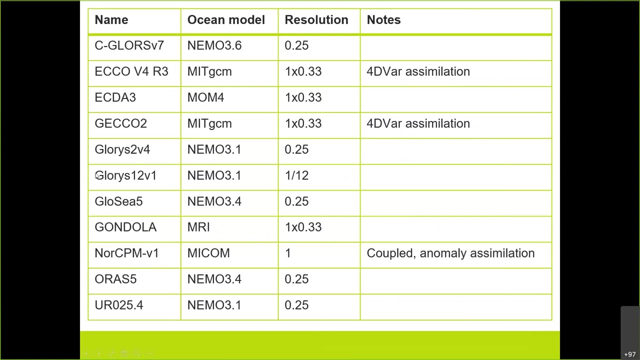 Echo and is and the and so Glossy 5. Or as 5 and the, What's the other? 1. And The seek laws as additions and the law and the glory space and solutions Available to download from the Siemens and website. 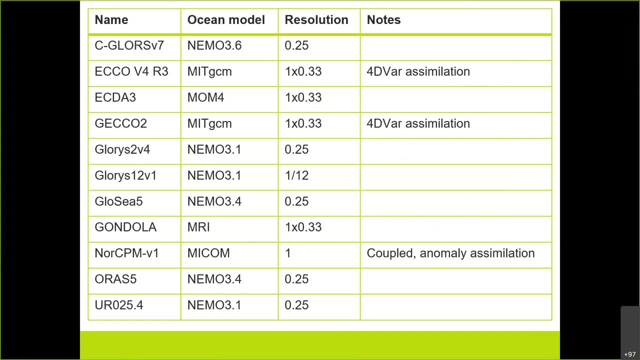 I think we'll take a few extra minutes to try to get through these questions. There is 1 from Bill John. Yes, since the models get the mock right about right at 26 North, do we understand why they all consistently underestimate the heat transport? 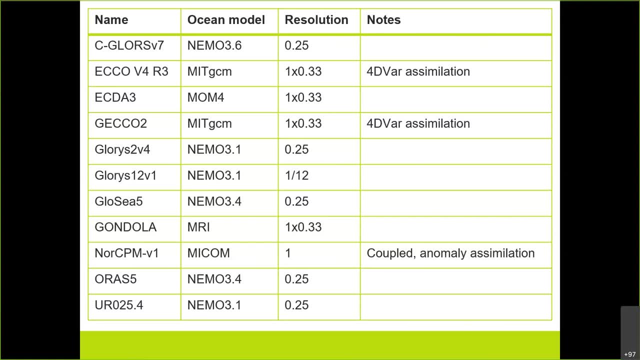 Um so, so we think it's a part of the. I know from other model studies. There's issues to do with how to do with the firmer client and also to do with getting the Getting the temperatures right in the boundary counts, I think. 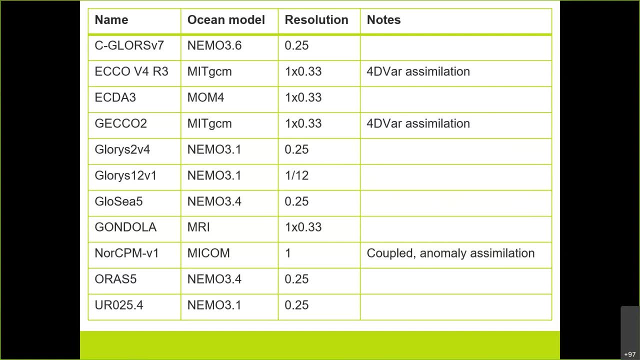 But I don't think anyone really knows Exactly what, with whether that's an issue resolution Or what. yes, I mean I guess. I guess the fact that the aim is generally too shallow might be playing a role as well. A question from a quick question: Do you think that data assimilated re analysis products? 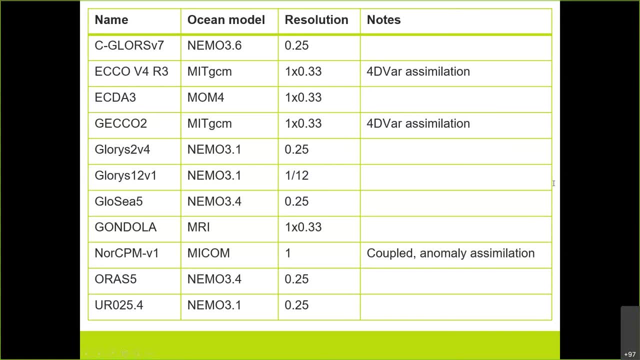 Are better than the surface forest model runs and reproducing the a mock time series. So, from what I have seen, The question. so in terms of the aim of 26,. no, I haven't seen any Surface force model runs, so they they can get the 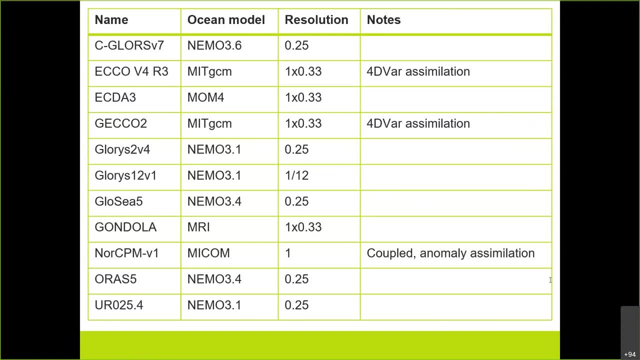 But I haven't seen anyone showing them getting the weakening trend Trend At all. so that seems to suggest that the analyses are doing that and we don't know this big question as to why they're doing that: What is it that they're assimilating? which is allowing them to do that? 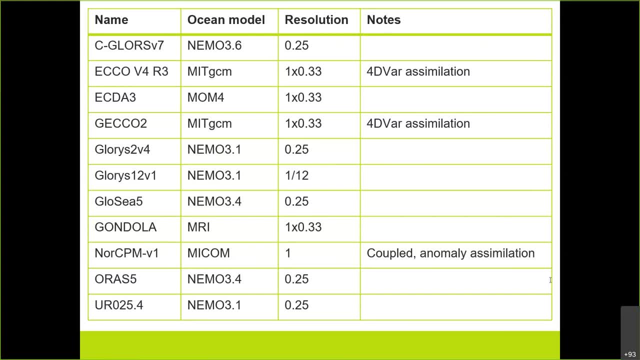 In terms of at 50 North. the force models all show show this weakening from from the mid nineties Which is very similar to what we're seeing in the analysis products. Go con did make a comment for simulations get the weakening. I believe. 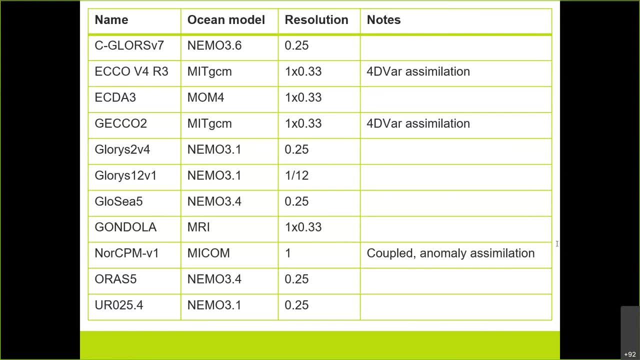 A question from John Hall. did your group attempt to quantify and compare a mock and density coordinates rather than depth space? So we only looks. so we looked to the Section, but only in a few analyses. So you appreciate that it's more complicated. 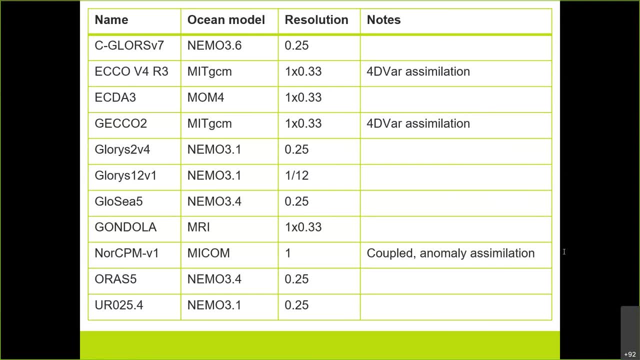 to calculate. We've got it in our reanalysis, but we didn't get anybody to calculate that. And a question from Ranellas Perez: Have you looked at whether there is a large spread in the reanalysis trends in the South Atlantic? No, is the answer. So this was the paper. 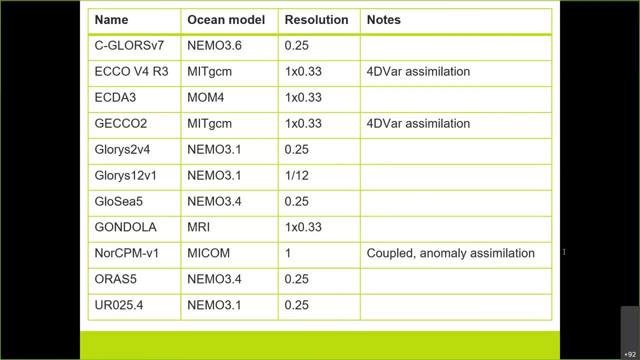 focusing the North Atlantic, so we didn't look at the South Atlantic. And then I know we have two audience questions still waiting. Shane, do you want to go ahead and ask your question? I don't hear you right now, Shane. are you there? All right, let's. 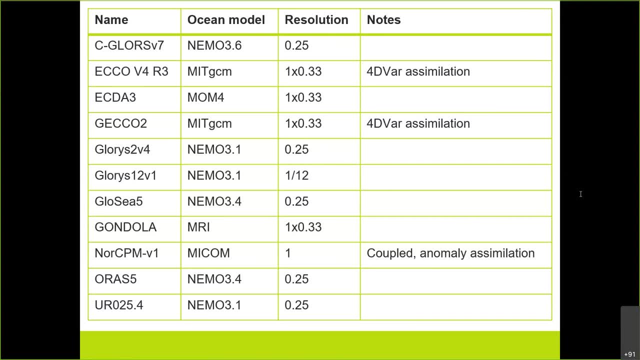 move on to Anish. for now, Anish, you want to go ahead and ask a question? Okay, sure Can you hear me, okay? Yep, we can hear you, Okay. Thanks for the very interesting presentation, Laura. My question was regarding what observations have an impact on the AMOC.